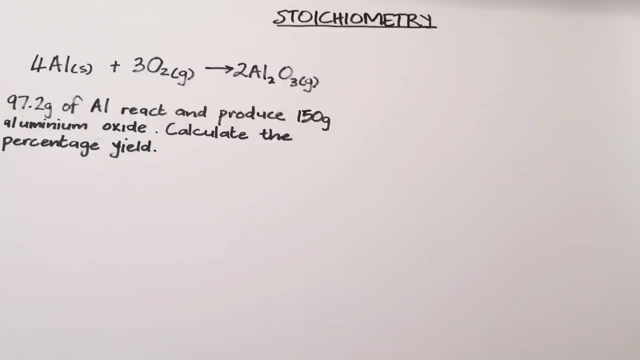 um, but also those who are doing their first year analytical chemistry. So, um, just enjoy the lesson And, obviously, if you haven't subscribed, you're more than welcome to do so. Welcome to the family and let's get into the lesson, Right? So I just wanted us to do this example. Um, we're in. 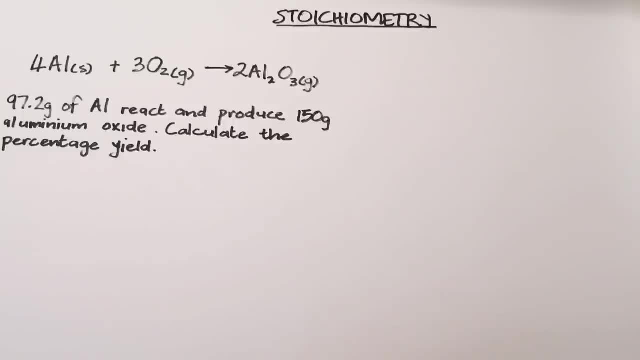 this um, four aluminium moles. Okay, So there's the reaction equation there. So that's four AL. all right, That reacts with oxygen and it gives us aluminium oxide. Now, if you haven't watched my previous videos on stoichiometry, perhaps it would be good to pause here and actually refer. 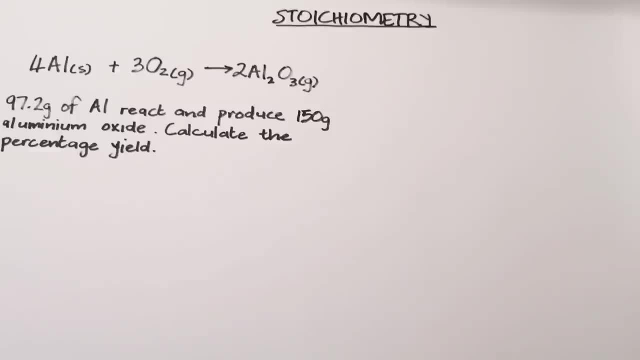 back to my lessons, uh, so that you can follow on, because I'm just going to build up on what we have done previously. Okay, So let's get into this question, Right. So they say to us: we've got 97.2 mole, uh, grams, rather, of aluminium. Okay, 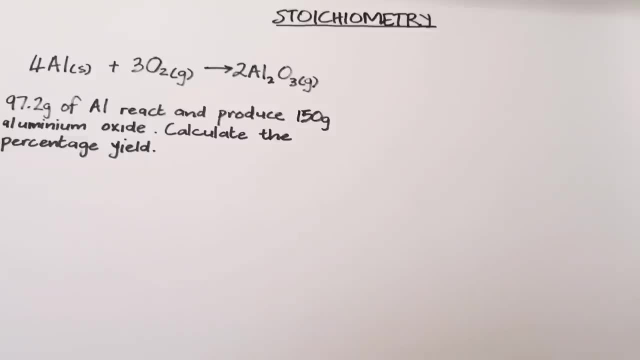 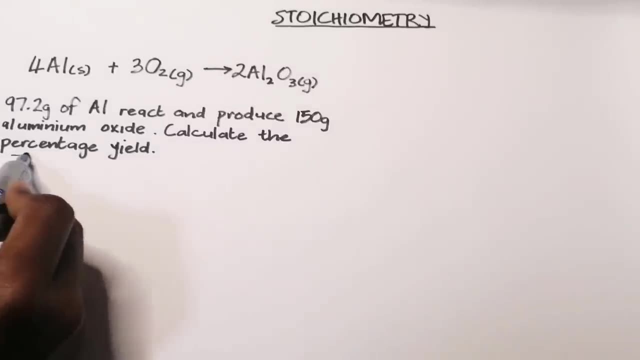 That react and produce 150 grams of um, aluminium oxide, All right. So they want us to determine or to calculate the percentage yield? Okay, Right, What is the percentage yield? Let me just explain that quickly. So essentially, when you've got uh, substances that react, okay, The ideal is that. 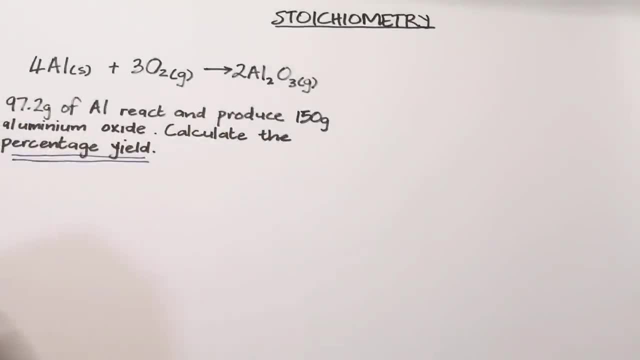 they are going to react completely And obviously they are going to give you a maximum amount of products. Okay, So if you take my analogy of um, you know flour and sugar, you know to make, um, uh, to bake muffins. So whichever one is, 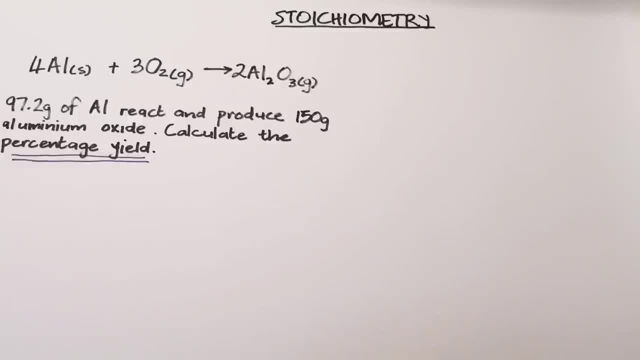 is limiting um um between the two reactants, your flour or your sugar, whichever one will limit the amount of uh cakes that you bake. All right, You, you obviously expect that you will make the amount of um uh cakes, uh, that you're going to make. So you're going to make. 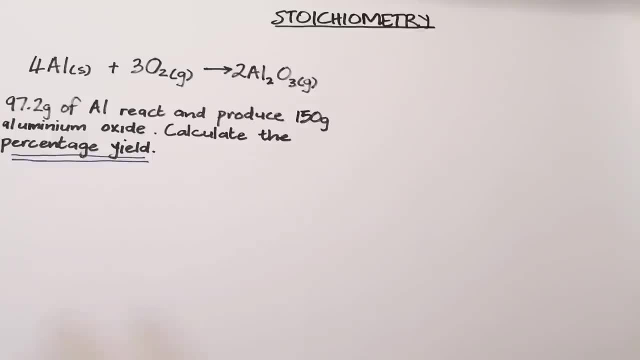 muffins. that are in relation to the limiting reagent. But in chemistry we sometimes find that that is not the case. We find that some substances react completely and some actually don't. Okay, For some or other reasons, because, uh, the rate of reaction decreases or uh, uh, you know for 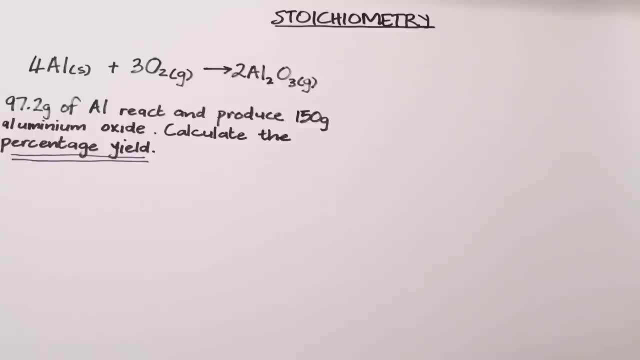 for for many other reasons. So, essentially, what we want to find out is what would be the percentage of the product that I get if I compare it with the ideal that I would have gotten. I hope that makes sense, You'll. you'll understand it as I, as as I explain it. Okay, So there's an. 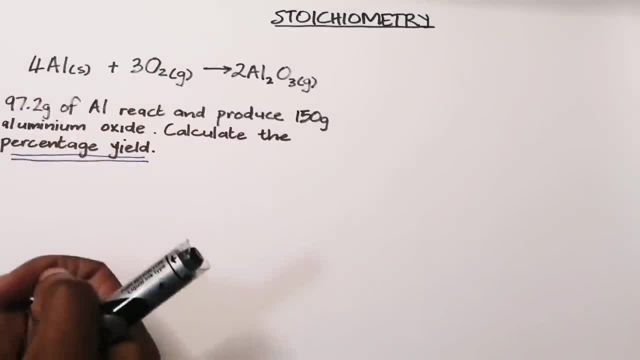 ideal amount that I would have gotten, based on my reactants, but then you find that that ideal is not met, but you actually come or fall short, uh, of the amount that you're getting. So you would have gotten okay. So, essentially, how am I going to get that? All right, Now let's do this. 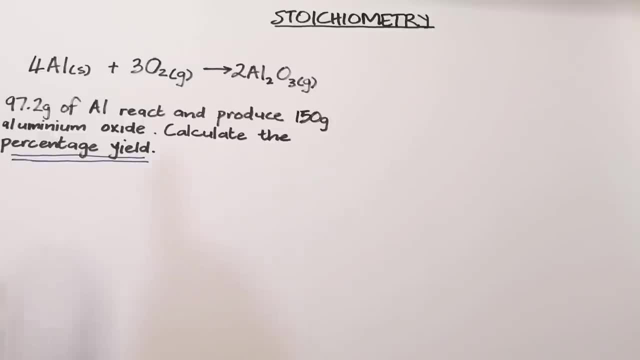 We're going to first determine, all right, based on the amount of reactant that I have. Okay, Let's assume that oxygen is an is in excess, even though they didn't tell us. So it means that it would be in excess, right? So it means that aluminum therefore becomes my limiting reagent. 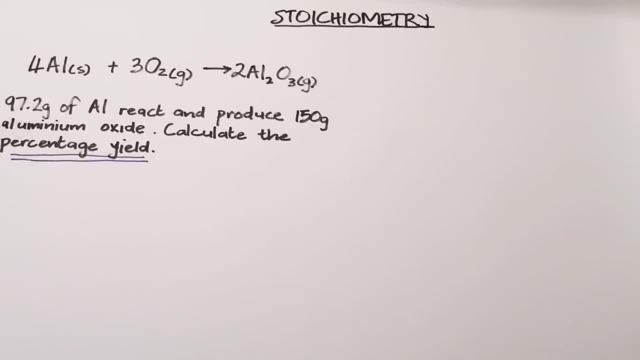 Okay, It is the one that is going to drive the reaction. It's the one that's going to determine the amount of product that we would actually, uh, receive at the end, right? So let me find out how much aluminum I have, And, given this amount of, 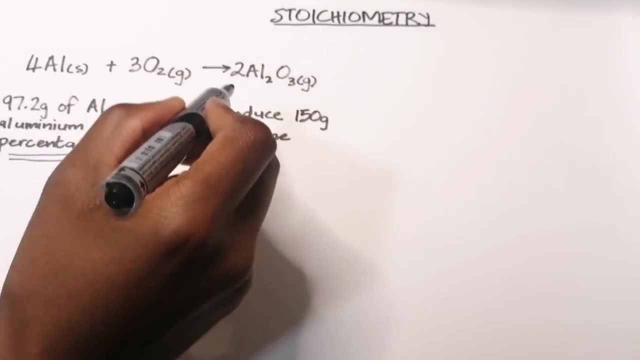 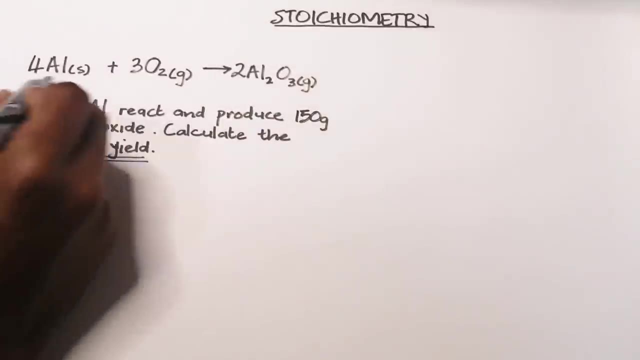 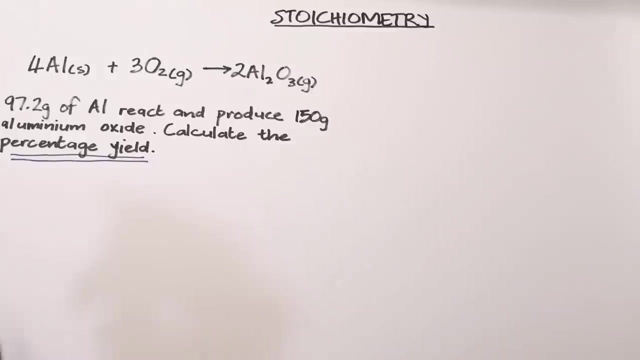 aluminum. how much, therefore, the aluminum oxide I ideally should be able to produce? Okay, So let's do that. So we're given the- uh sorry, the mess. Okay, So you, I, I suppose you know the drill by now. So we first convert from mess to molar mess, right? 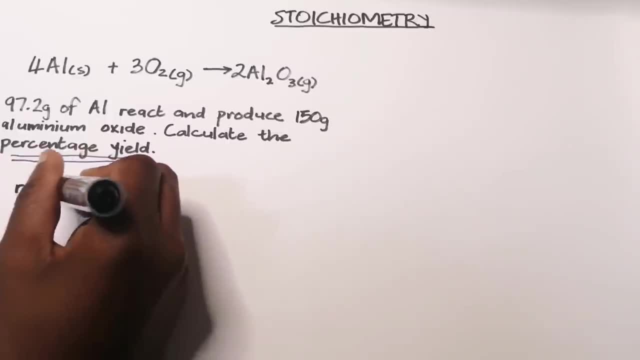 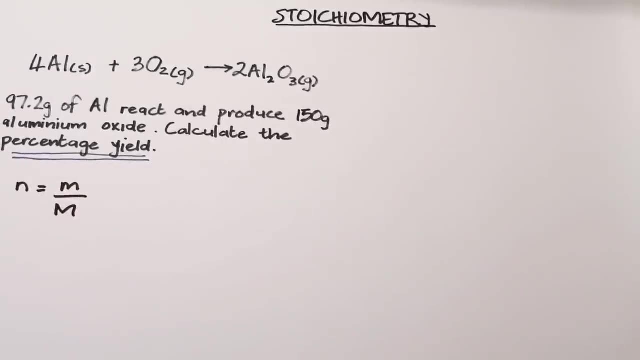 So we're going to say, okay, number of moles. This is going to be mess divided by molar mess. If you don't mind, I'm just going to use a different color, Okay, So that you can tell between the question and the answers, right? So this is number of. 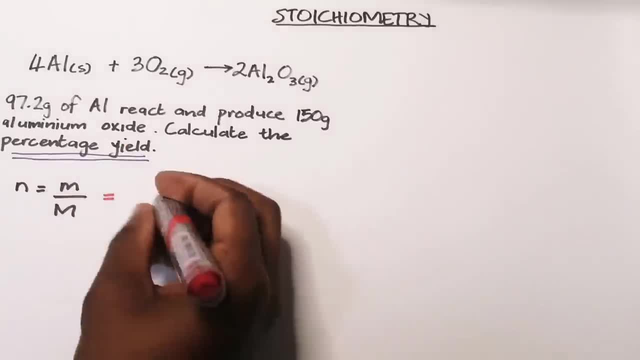 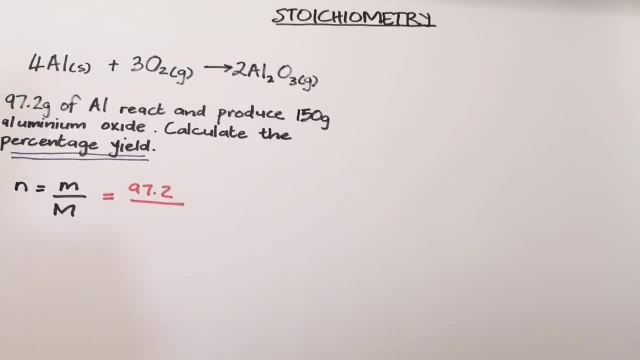 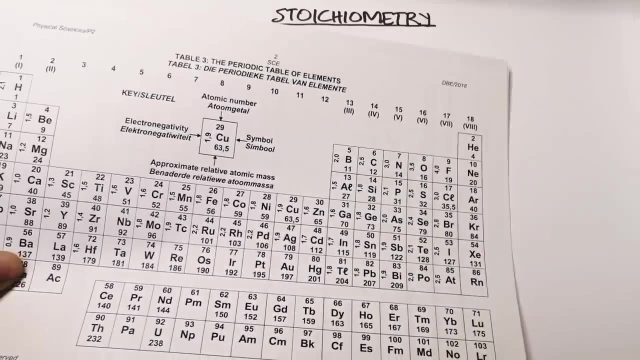 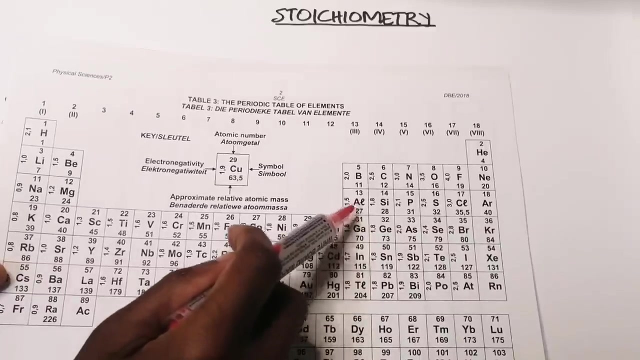 this by now. if you haven't watched my previous videos, please refer back to them. So we're going to go to the periodic table to check what is the molar mess or the relative atomic mess of aluminum, right? So if you look at that, uh, there's aluminum over there. Okay, Element 13,. 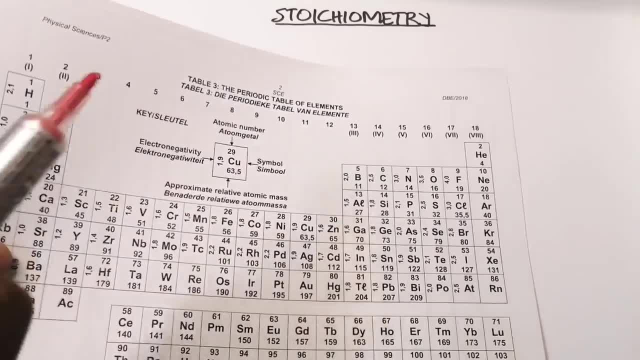 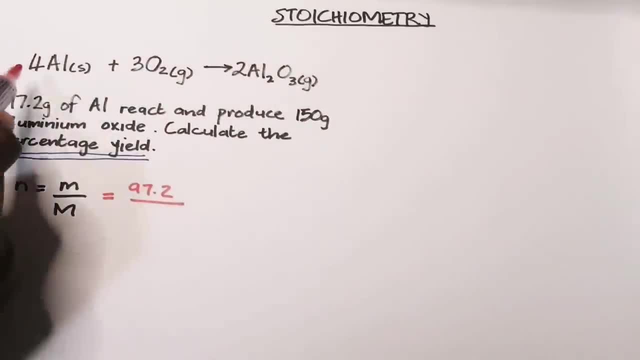 it's 27 grams per mole. Okay, Now, please remember, ladies and gents, it's just the element aluminum and you are not supposed, when you calculate molar mess, you are not supposed to use the stoichiometric coefficient. Okay, So in this case it's going. 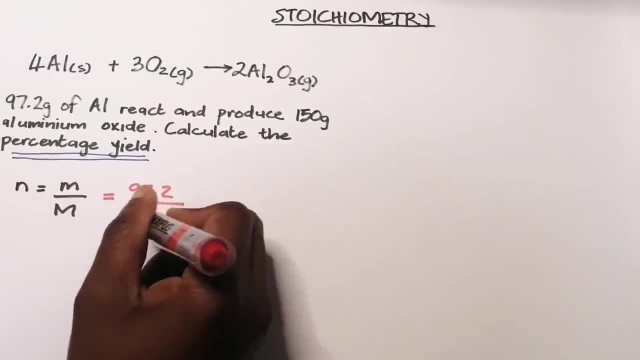 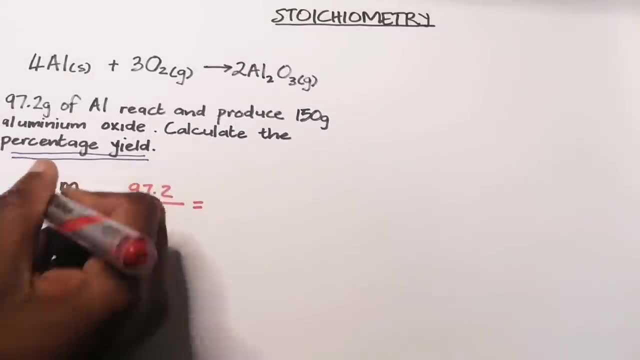 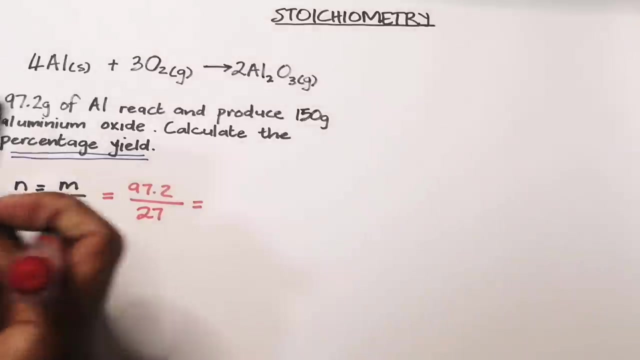 to be the molar mess. We said that molar mess is 27.. Okay, So let's find out how many moles of aluminum In fact. let me just write that there so that you know exactly what I'm doing. I'm looking for the number of moles of aluminum. Okay, So let's just put that in the calculator. 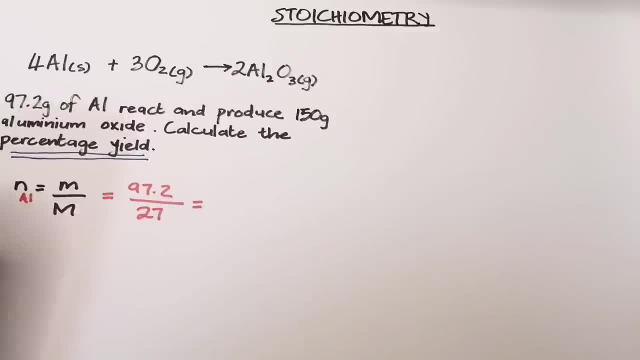 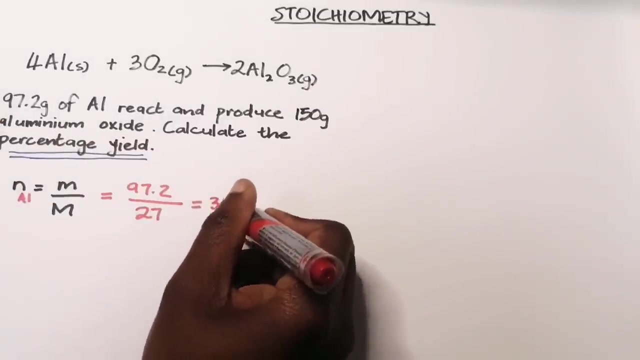 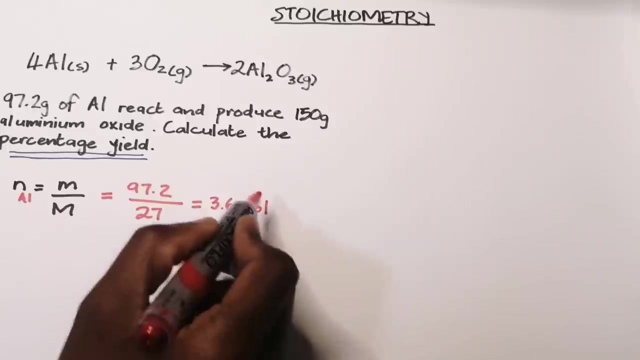 there. Uh, so I've got 97.2, and, and I divide that by 27.. Okay, So I divide that by 27.. Okay, So I get 3.6 moles. So, ladies and gents, I get 3.6 moles of aluminum. Okay, But remember our process. 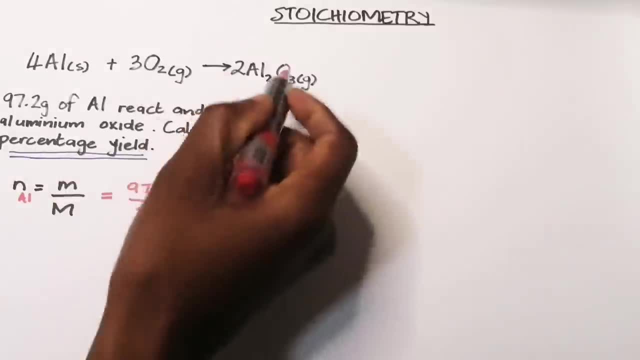 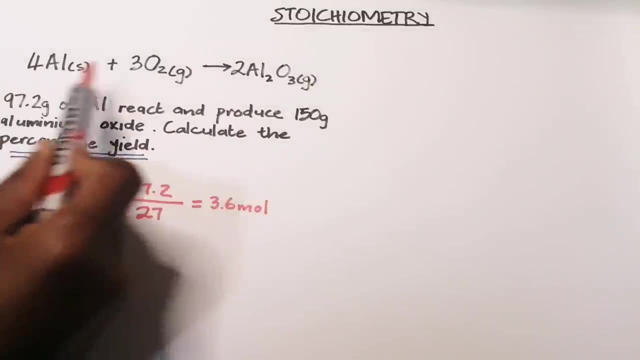 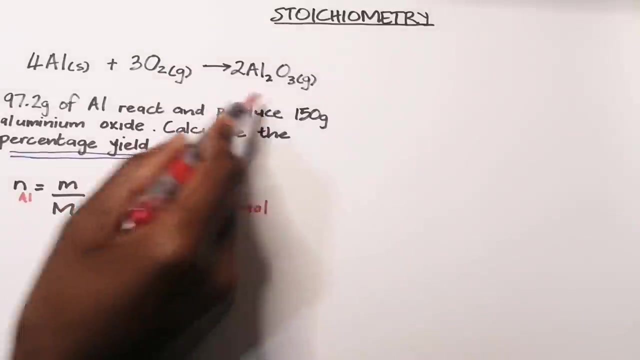 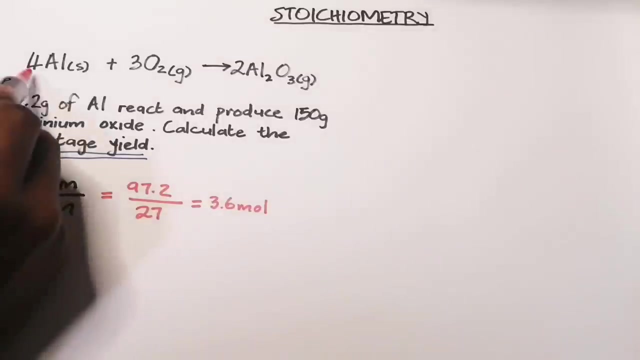 we said we start from moles, then we use stoichiometric coefficients, isn't it Okay? So now I'm going to use my ratios to actually determine, ideally, the maximum amount of aluminum X or oxide that I should actually be able to uh to to produce Right? So let's start there. So we 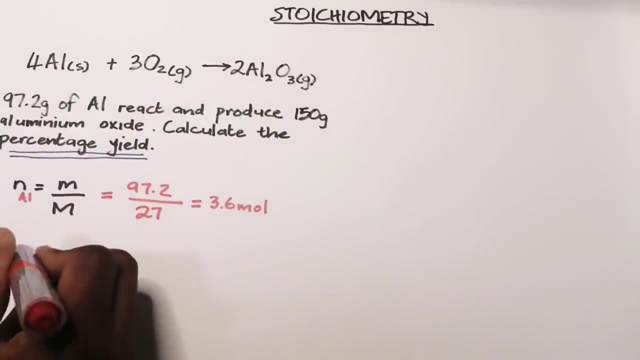 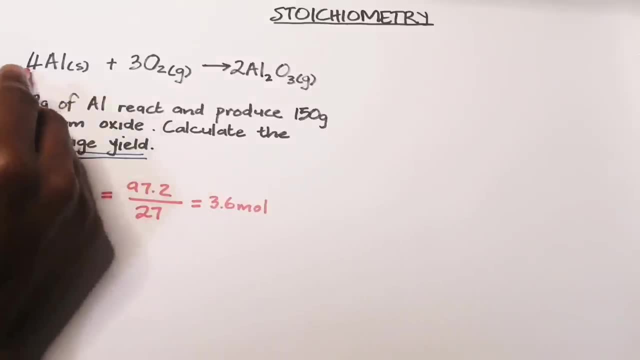 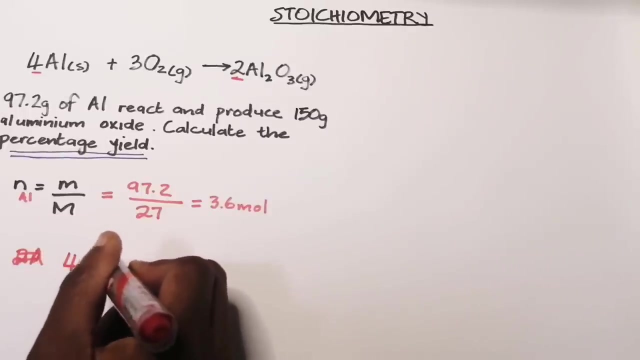 said, we always start at our reaction and I'm going to say for every two moles- uh, sorry, for every four moles, Sorry about that. So for every four moles. that's my, those are ratios, right. so for every four moles of aluminium, why am i using aluminium? that's the one that i 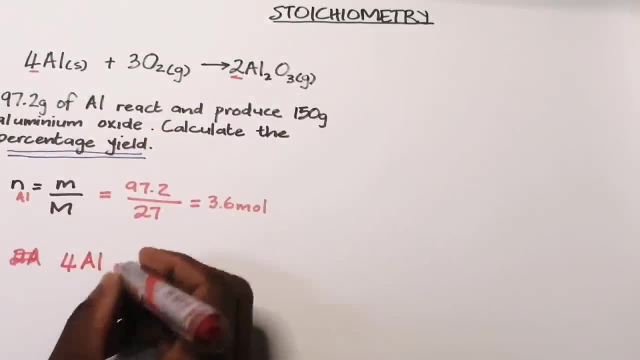 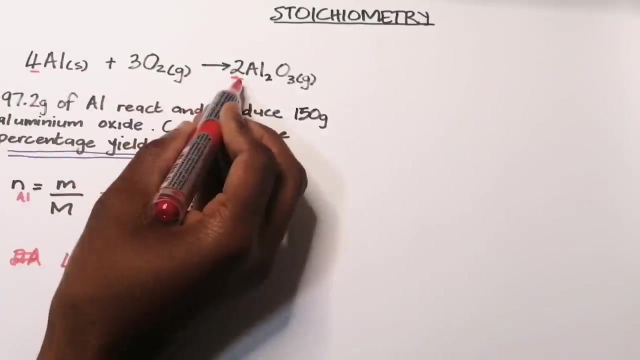 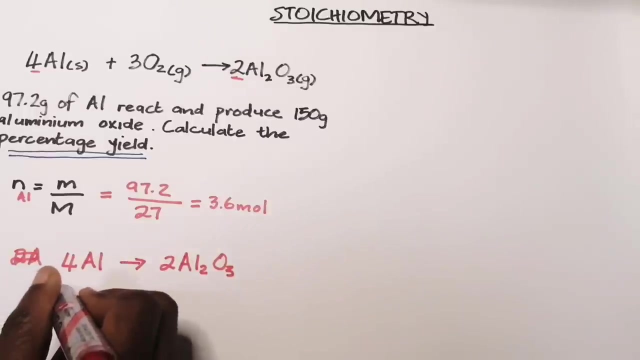 have? okay, and i want to determine aluminium oxide. so for every four moles of aluminium, i will produce two moles of aluminium oxide. okay, right, so that's according to my ratios there. okay. now let's get to this one here. okay, but here i've got 3.6 moles of aluminium, okay. so if i have 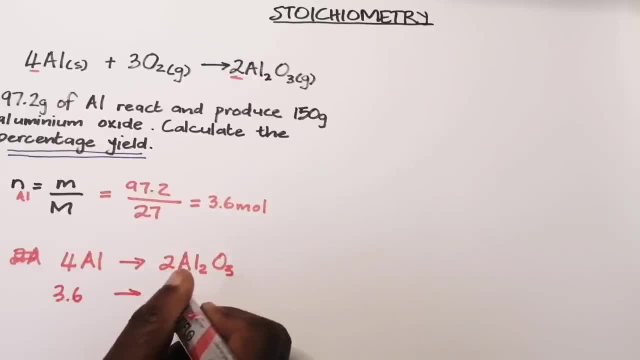 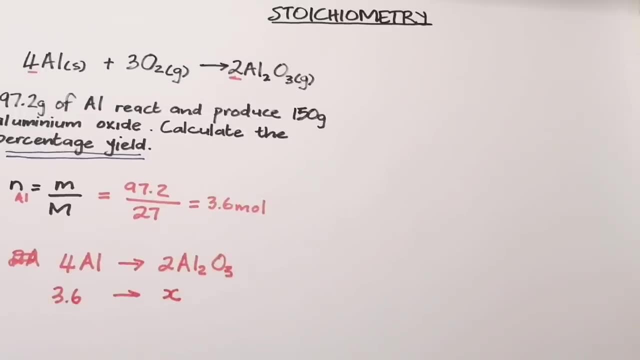 3.6 moles of aluminium. how much of aluminium oxide am i going to produce now? please allow me once again. i'm not going to write out aluminium and aluminium oxide again, but I just want to show you that I've written aluminium on the left and the moles of aluminium. 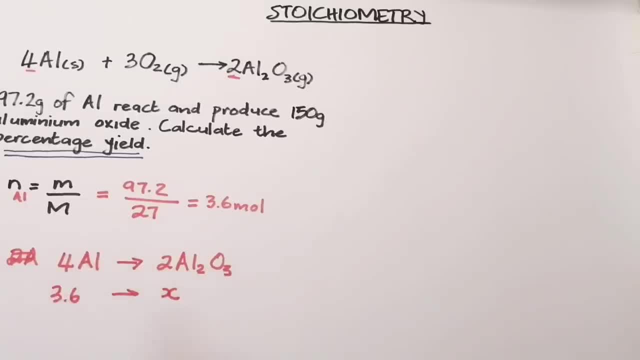 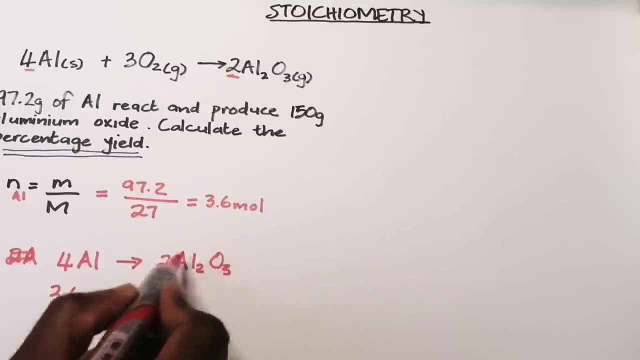 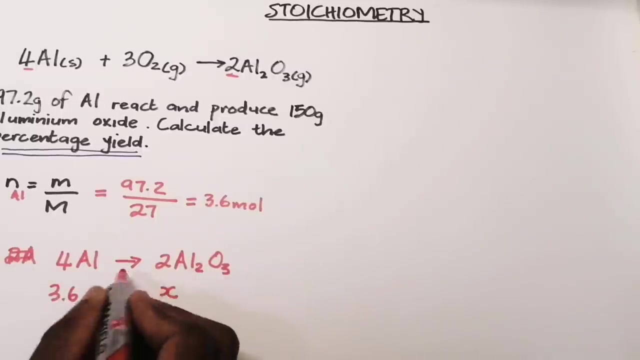 I also have them on the left hand side. So same things on the same side. That's the rule, Okay, That's. we call this ratio and proportion, right? Okay? So aluminium oxide: that's the one that I want to determine. I start with my ratio and I want to determine the amount that I will have. 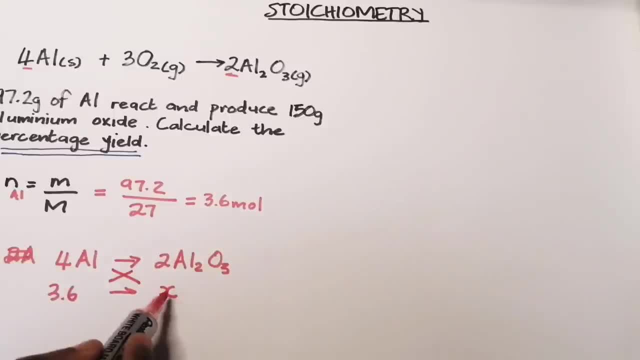 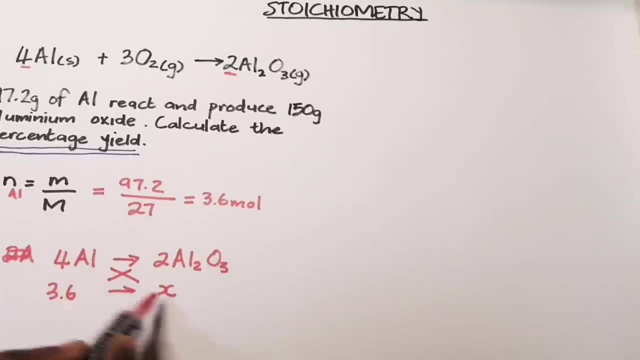 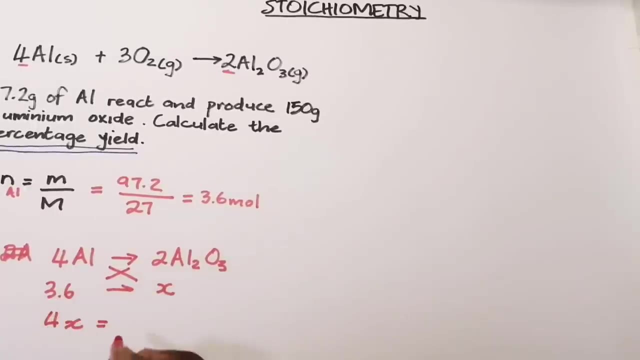 at equilibrium. So now let's cross multiply. Okay, Remember I said when we cross multiply we're just going to take the molar ratios. Okay, The mole ratio. So that's four times X. that will give me four X, which is equal to 3.6 multiplied by two. Okay, That should give us. 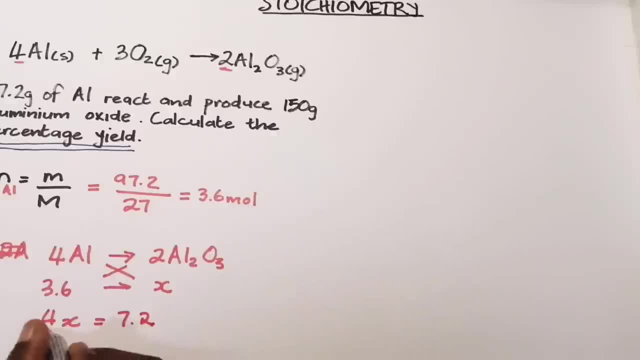 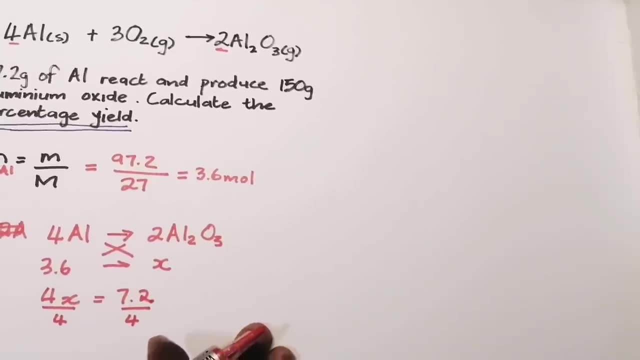 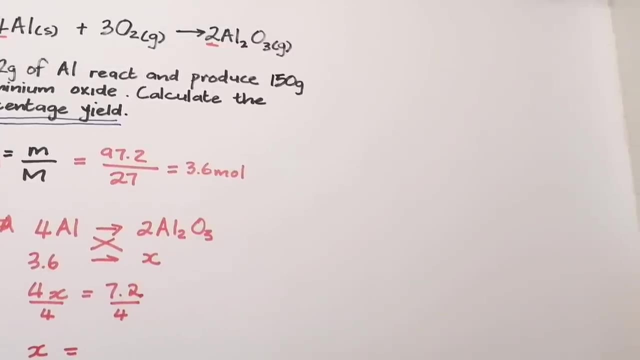 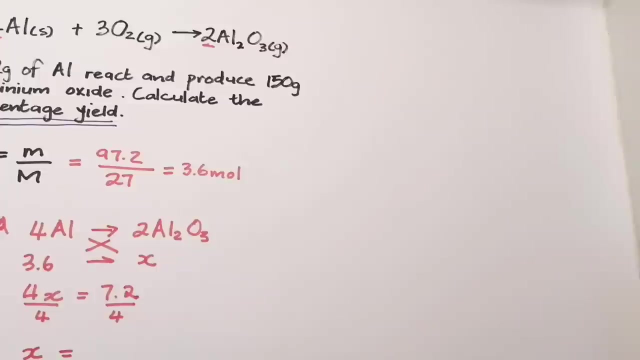 7.2.. Okay, Divide that by four. Okay, On both sides, And what you- I'm just going to raise that a little bit- Okay, So what I'm going to get there, Okay, So that's 7.2 divided by four. So that's 7.2 divided by four, And what we get is 1.8.. Okay, And it would 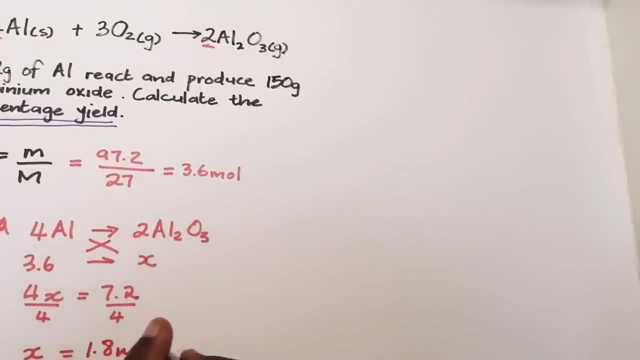 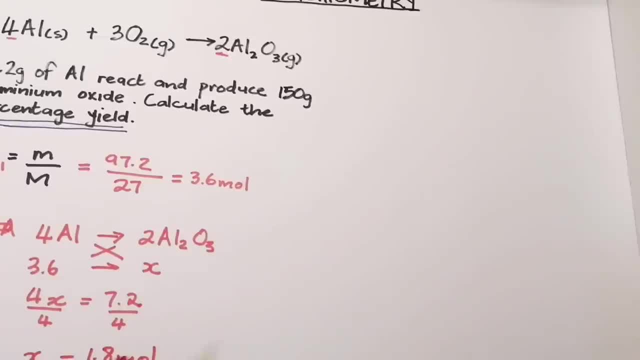 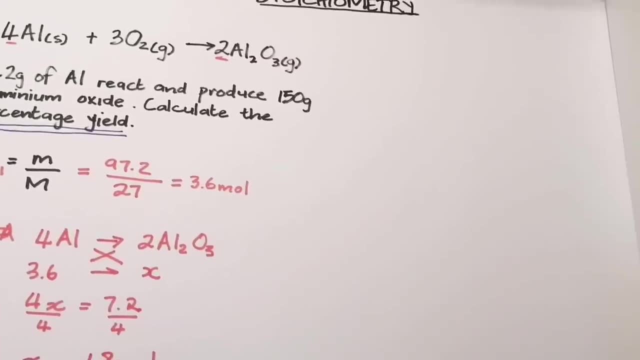 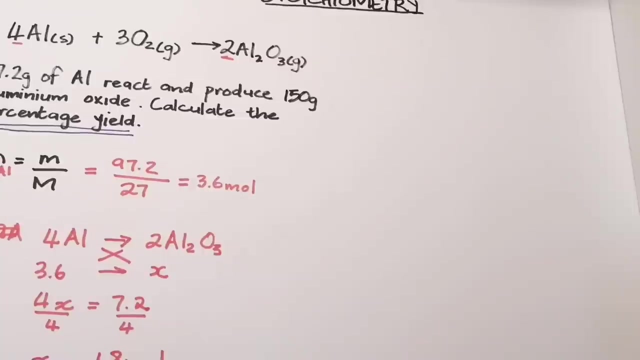 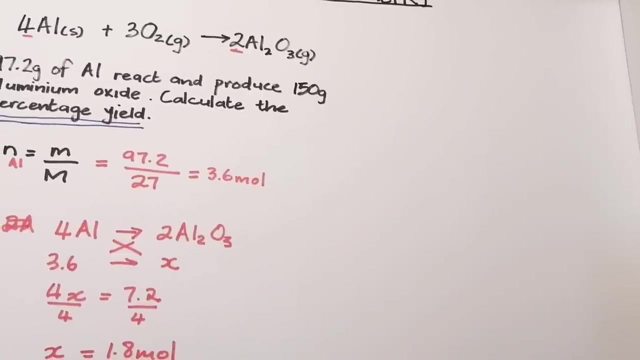 able to see this right at the beginning, Right? So I gave an amount of 97.2.. I was given an amount of 97.2 moles of aluminum, Okay, And we determined from that the amount of moles of aluminum oxide. 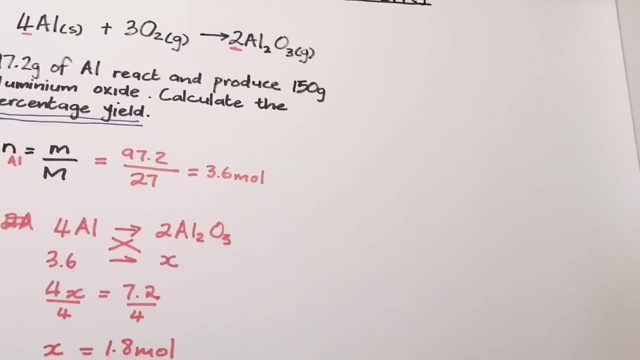 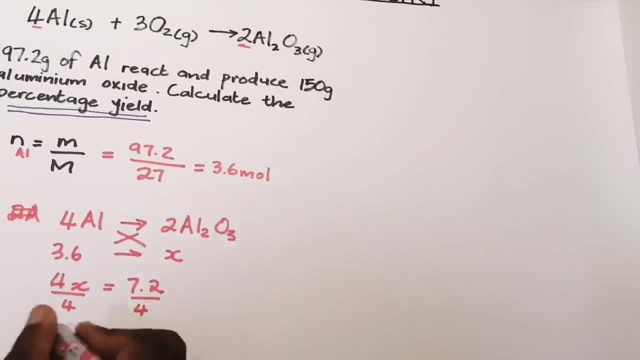 that we would ideally be able to get. So we determined from that the amount of moles of aluminum oxide that we would ideally be able to get. Okay, So now I want you to note what did I have, or what do I have right there? These are the moles of aluminum oxide that I would be able to. 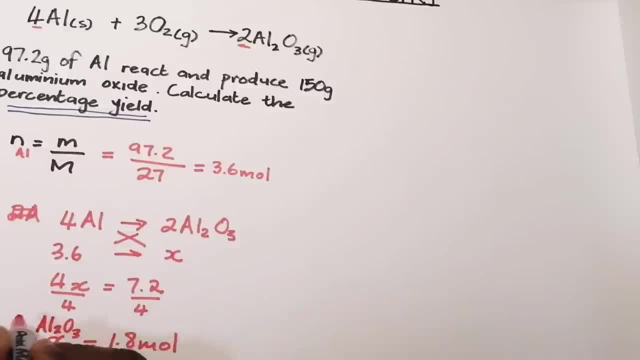 produce Right. These are the number of moles of aluminum oxide that I would be able to produce Ideally, if I'm able to use up all of the aluminum that I have Right, But now, according to that, I only was able to find only 150 grams. 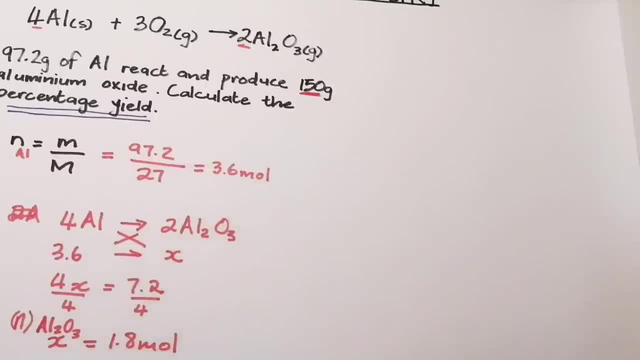 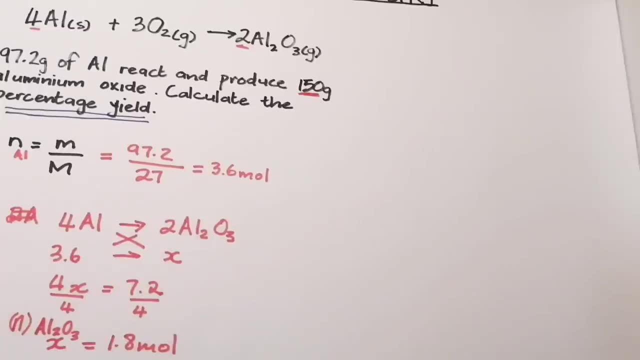 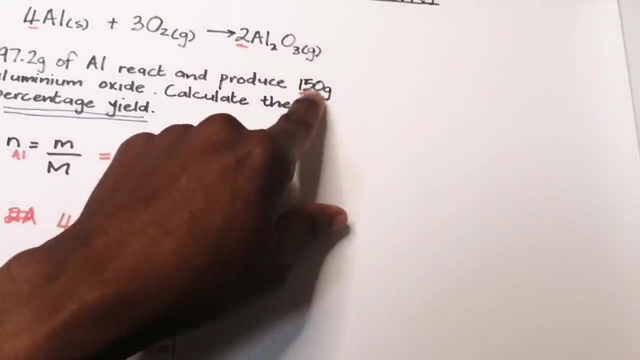 of aluminum oxide. Now there are two ways in which we can do that. We can either do that by using grams or we can stick to moles. Let me start with the one where we use moles. So these are the ideal moles of aluminum oxide, Right? So let me do this. Let's find out how many. 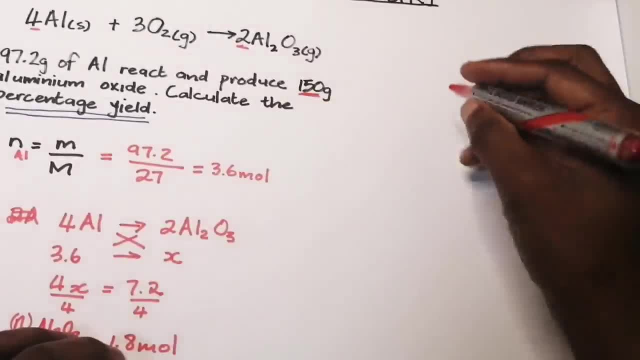 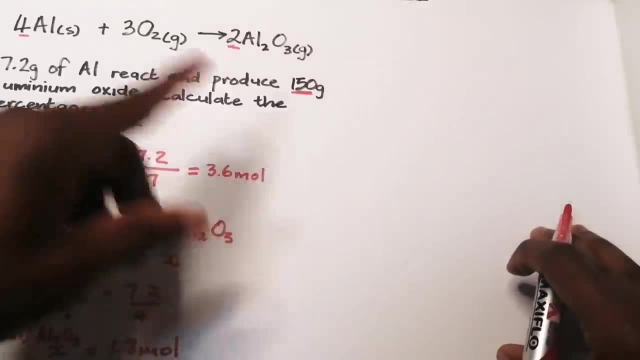 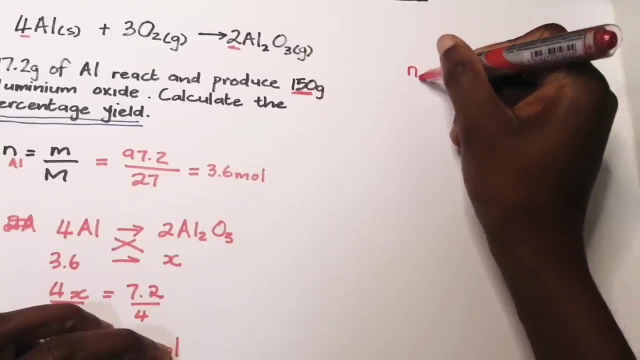 moles we will actually get. Okay, So those are the actual moles that we would actually have produced if we use from the actual reaction. Okay, So I'll say: okay, we want to find out the number of moles, the actual moles of. 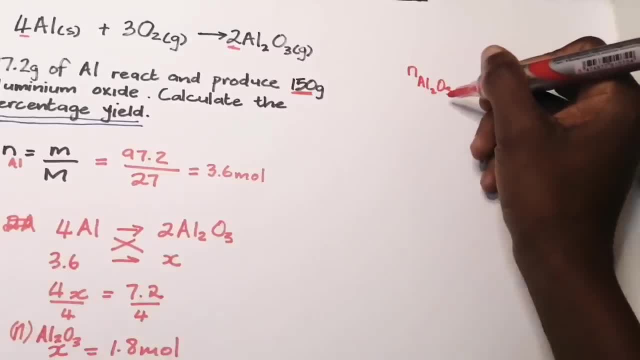 aluminum oxide. Remember, these ones are the ideal moles, These 1.8 moles, These are the ideal, These are the actual moles. Why? Because they told us we produced 150.. Okay, So, number of moles. 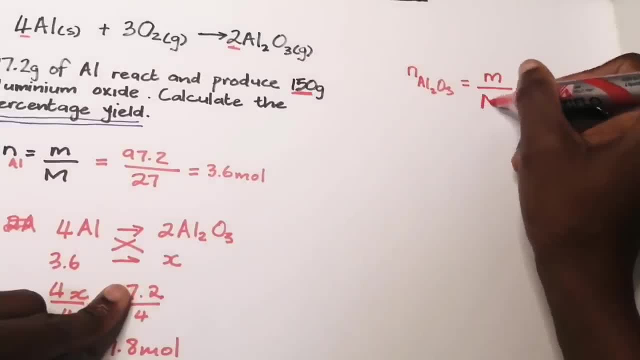 that's mass divided by molar mass. Okay, So mass, that's very easy, That's 150. We were given that, Okay, And we divide that by the molar mass of aluminum oxide. Now, please, I want you to note. 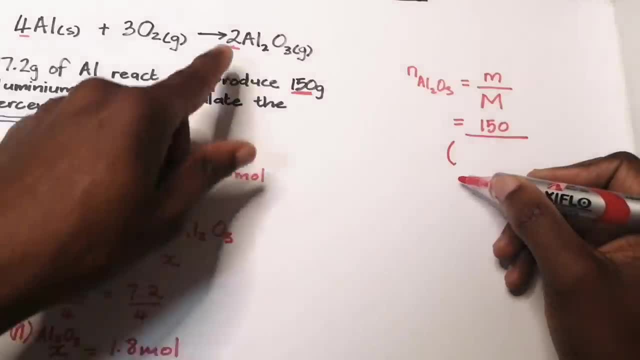 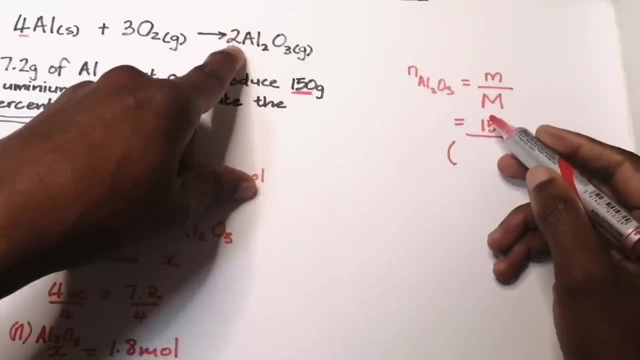 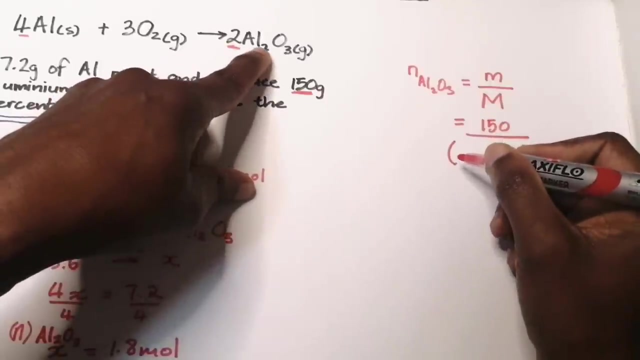 ladies and gents, I'm going to do it over here. So remember, when you calculate a number of rather molar mass, you do not use the stoichiometric coefficient, You don't use that number in front there, Right? So we're just going to look at aluminum oxide. So it's two atoms. 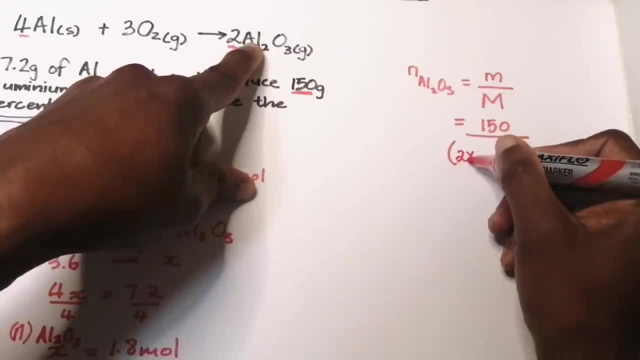 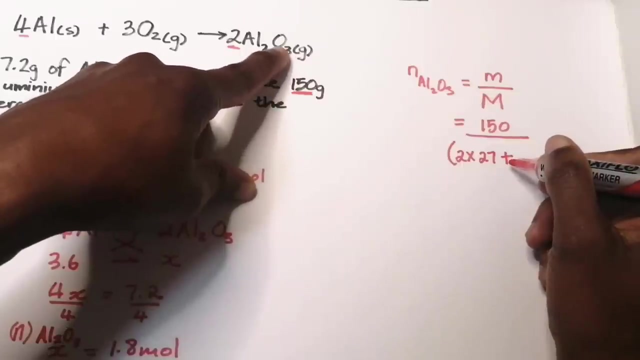 of aluminum. So I'm going to say two multiplied by. I'm multiplying because we've got two of them, So two multiplied by aluminum. we said aluminum is 27 from our periodic table, plus three oxygen atoms. right, We've got two aluminum atoms. 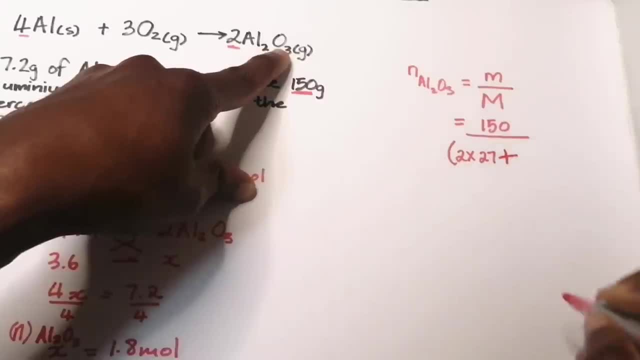 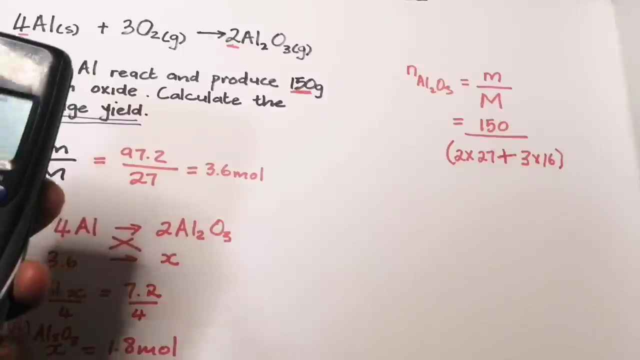 we've got three oxygen atoms. Note I'm adding: Okay, So plus three oxygen atoms, and that's three multiplied by 16.. Okay, And let's determine that. Okay, So I'm just going to actually just calculate everything all at once. Okay, So I'm just simply going to say 150.. 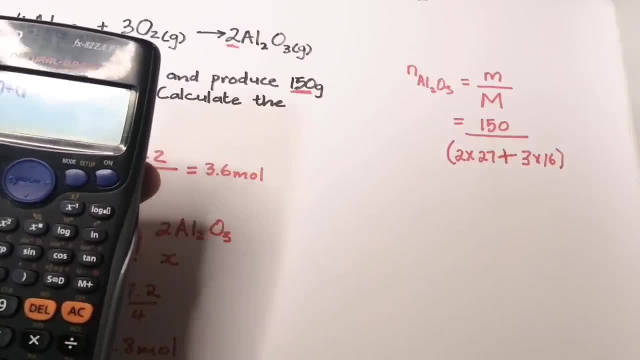 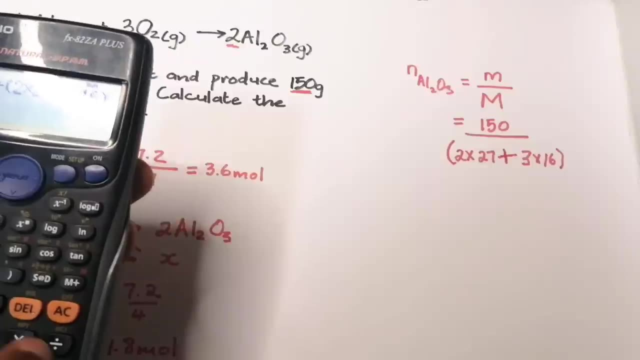 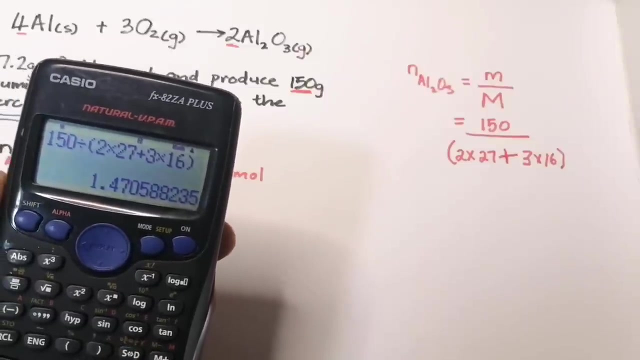 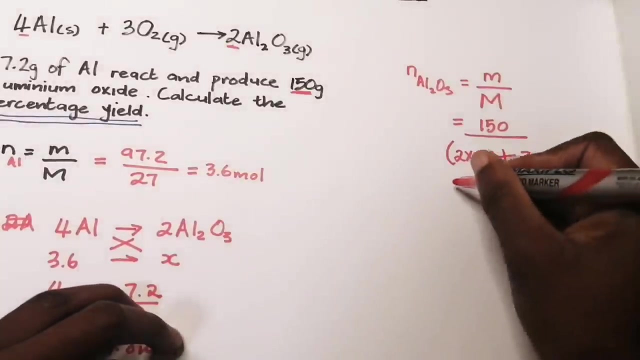 Okay, 150 divided by Okay, So we've got two times 27,, plus three multiplied by 16.. Okay, So we've got everything there. Okay, So that gives us 1.47 moles. Okay, So the actual moles of aluminum oxide that we produce is 1.47 moles, Right? So these are the number of 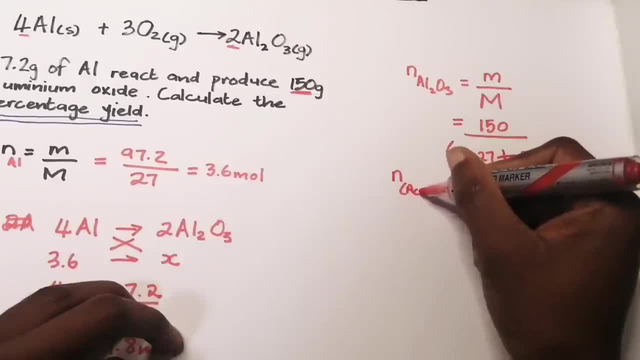 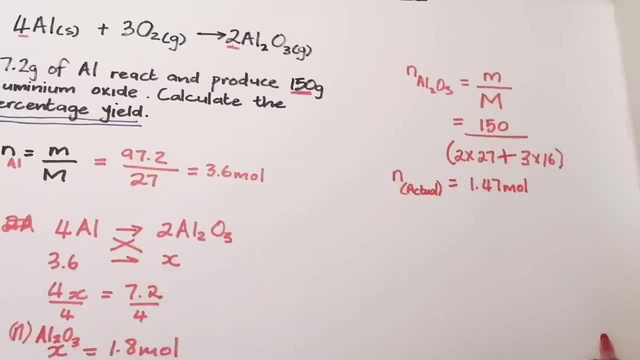 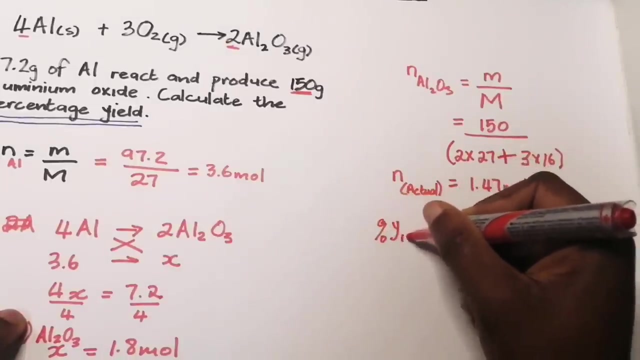 moles of aluminum. All right, Let's just write the actual. Now let's get to the last part of it. Okay, So how, then, do we determine the percentage yield? Okay, So, the percentage yield. ladies and gents, all that you simply do for the percentage yield, what you'll always do, is that you will take. 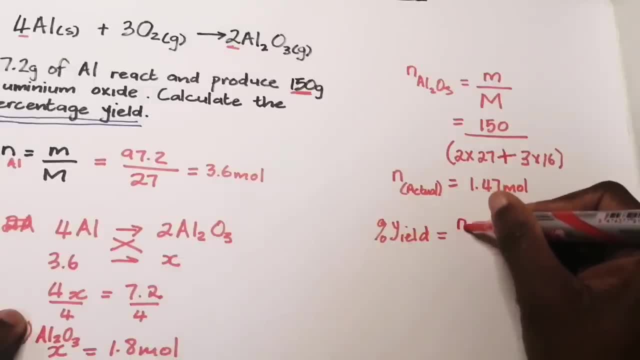 the number of moles, Okay, That you have actual. Okay, The actual number of moles divided, rather, by the number of moles that you have. Right, The ideal, The ideal number of moles, Are you with me? Okay, So that's the actual number of moles. 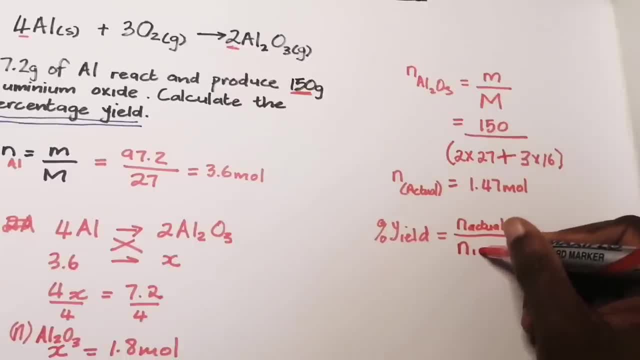 divided by, you can say divided by the ideal number of moles. Of course, to make that a percentage, we have to multiply that by 100.. Okay, All right. So in this case I'm going to say all right. what's the actual number of moles? That's 1.47. 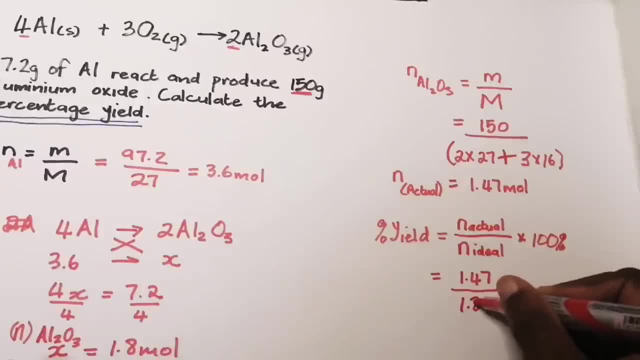 divided by what's the ideal number of moles. We said that's 1.8.. Okay, Right, And you can multiply that by 100.. And that will give us the percentage. So I'm going to say 1.47 divided by. 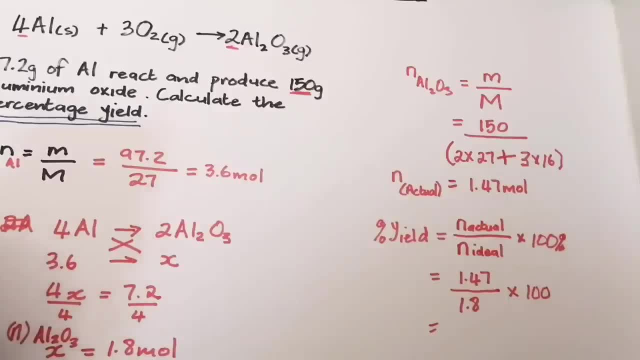 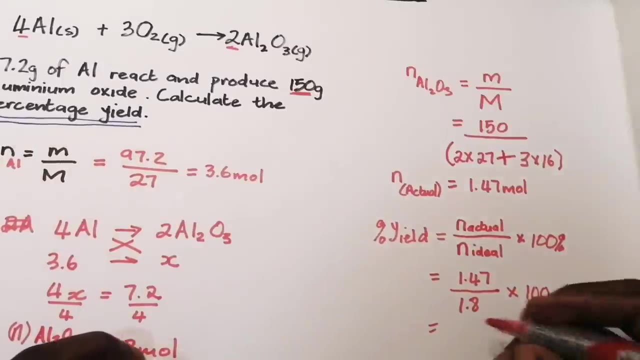 1.8.. Okay, Right, And what I get there is well, I'm just going to round it off to about 82%. Okay, So I get 82%. So it means that my percentage yield is 82%. It means that, of course, there are ways. 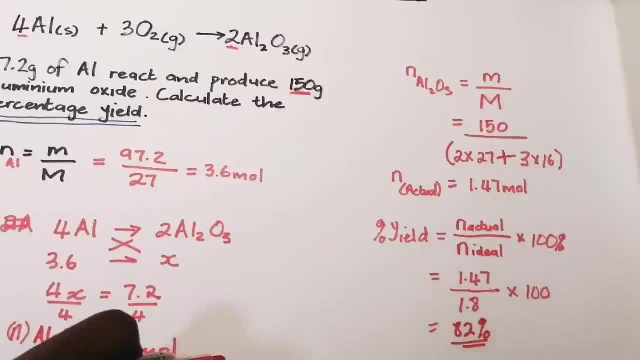 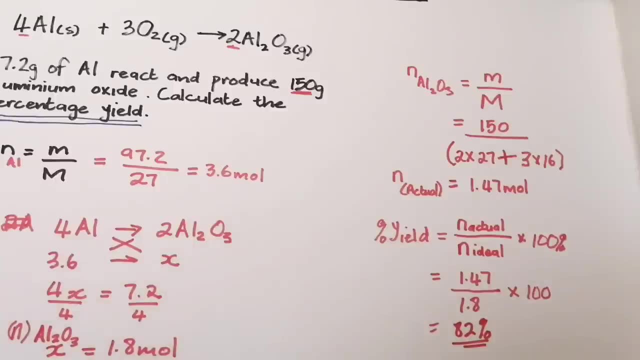 in which you can try and improve that. Okay, But that's a relatively good percentage yield. So obviously, for those of you who are doing analytical chemistry- you would be- you would know what are the factors that affect a reaction And obviously you would know how to improve that. 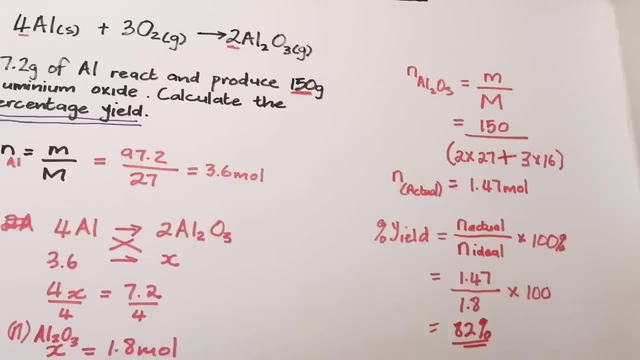 percentage yield. So that's a relatively good percentage yield. So obviously for those of you who are doing analytical chemistry- you would be- you would know how to improve that percentage yield. I hope that makes sense, Right? Just to show you another way before I just finish off. 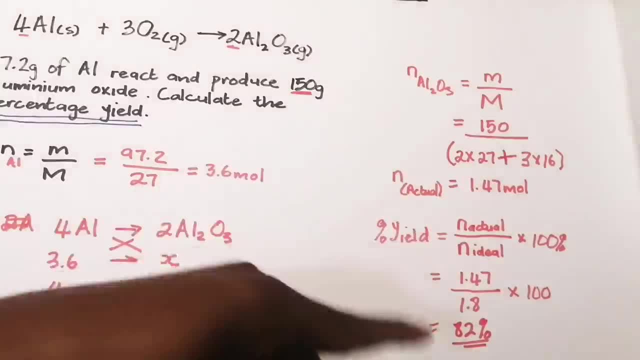 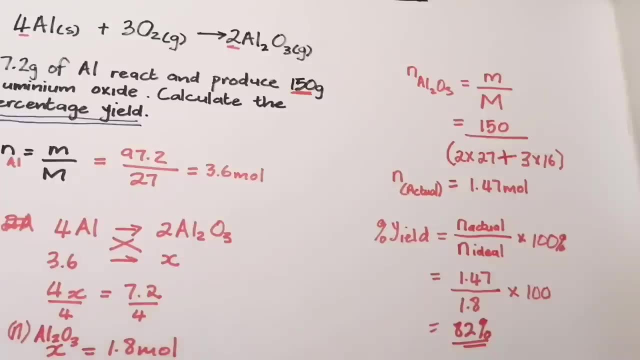 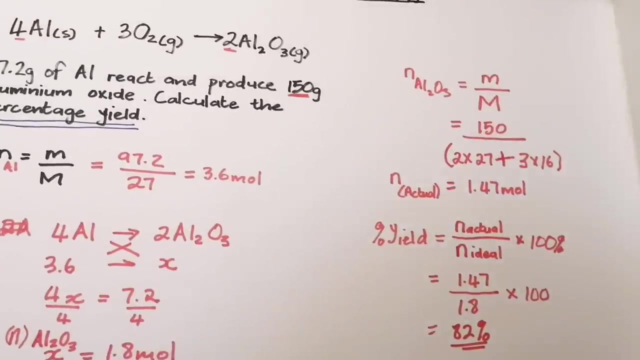 with this example, All right? So we could have done this using MESS, Okay, Just to show you that quickly. So if I use MESS in this case, okay, I'm just going to write over it there. Okay, All right, Perhaps I should use just another. 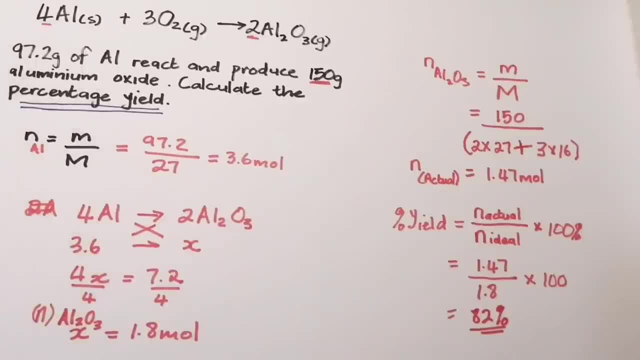 space there, Right? Yeah, Let's just use this one here, Let me just take another, All right. So what I could have done is to say: look, I'm still looking for percentage yield right Now. if you remember, what we did was we took the number of moles, we determined the number. 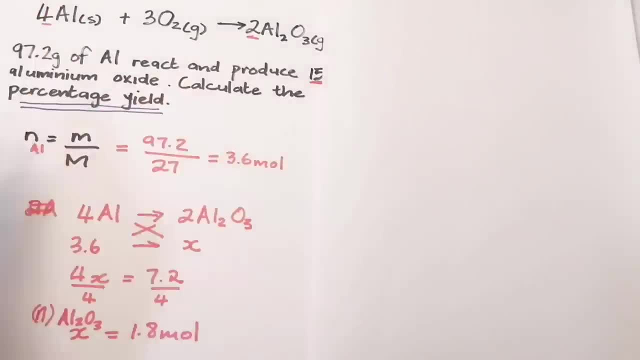 of moles. Remember, you can only do stoichiometric, or rather ratio and proportion when you use your stoichiometric coefficients. You only use that with number of moles, right? Remember, at age we said number of moles are to chemistry, what cups are to the kitchen? right, So in the kitchen. 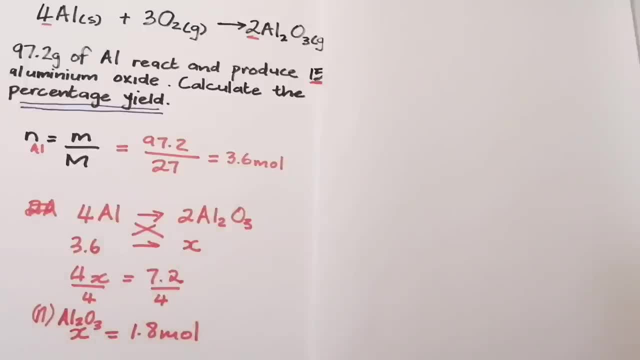 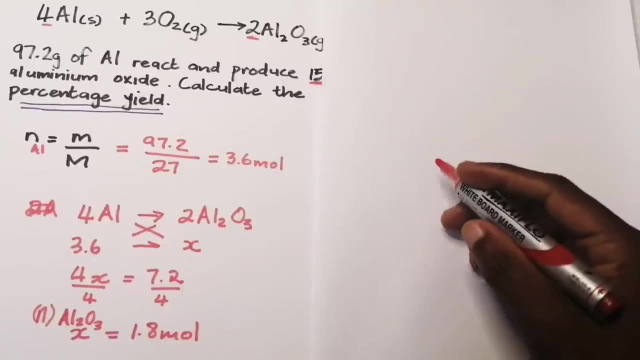 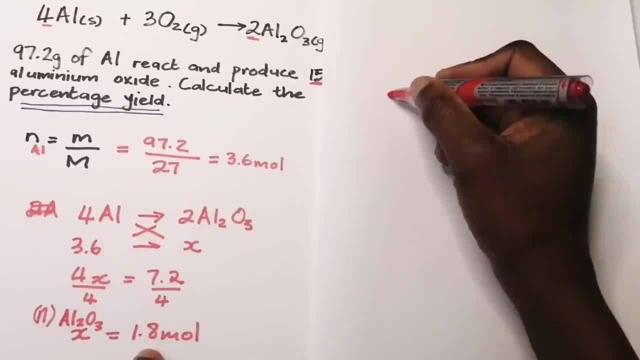 we convert to cups, but in chemistry we convert into moles. Okay, Right, So look at this, Just to show you how we could have actually done the very same thing. Okay, So I found out, I found the number of moles of aluminum right. And then we use that stoichiometric coefficient to convert to. 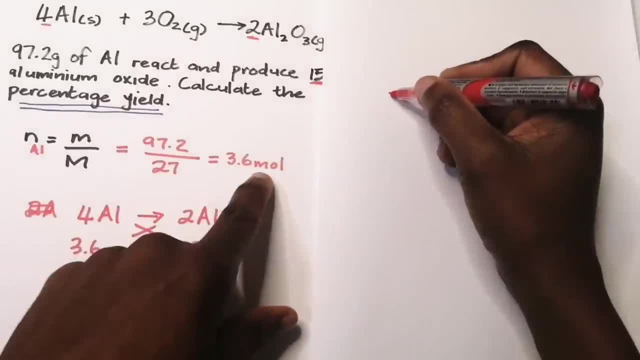 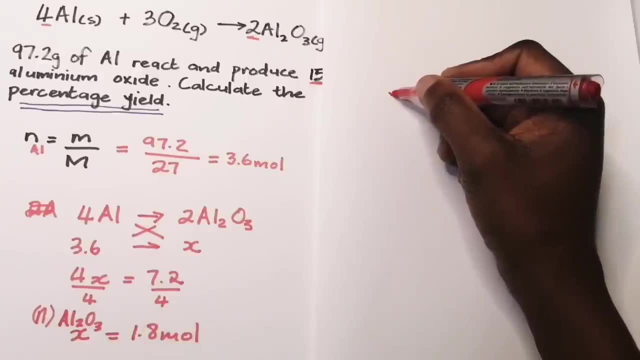 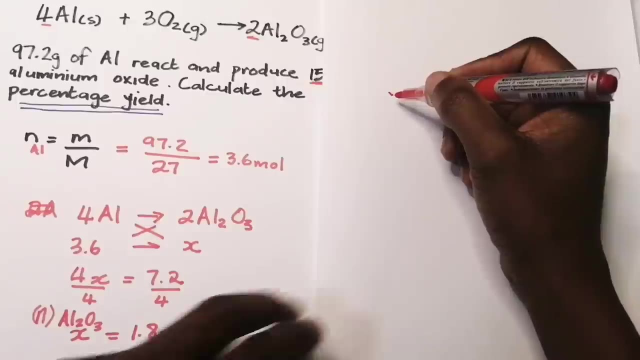 stoichiometric ratios. Okay, We found the number of moles of aluminum. We use that stoichiometric ratios. We found out the ideal number of moles that we would be able to produce. Okay, So as a result, I can take these number of moles and find out the mass. So I can say, well, how do I get the? 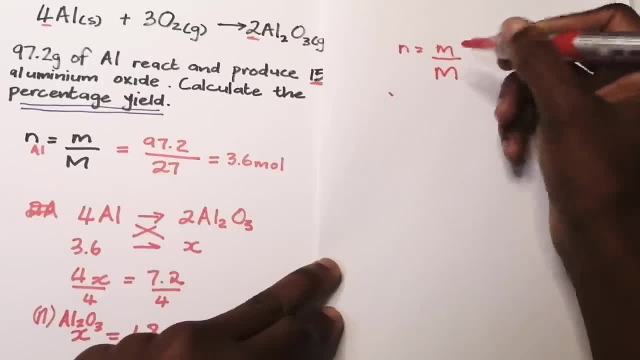 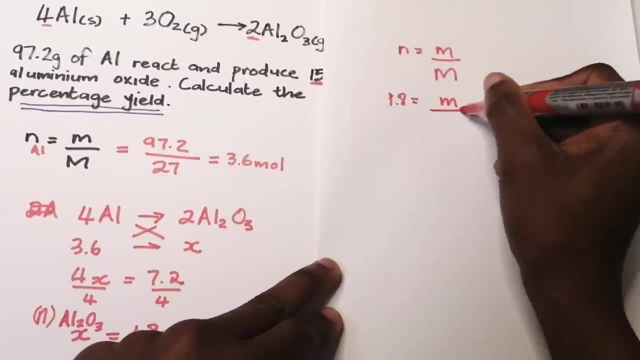 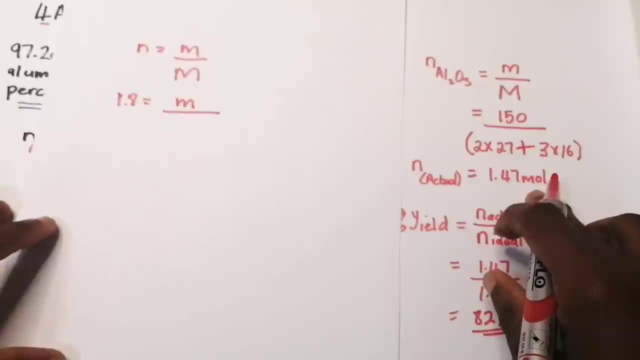 mass of aluminum that I'm going to produce. Well, I've got the number of moles, which is 1.8.. Okay, I want the mass. Okay, See, now it's working against us that we didn't actually calculate that molar mass there. 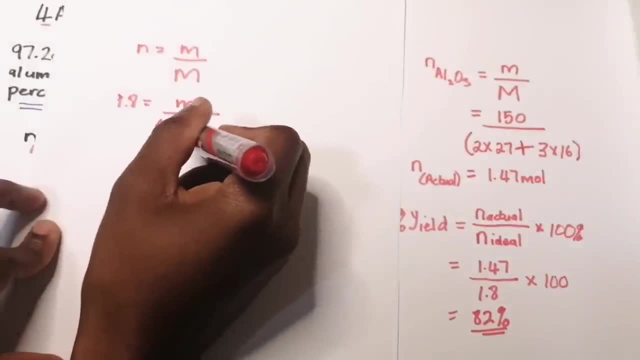 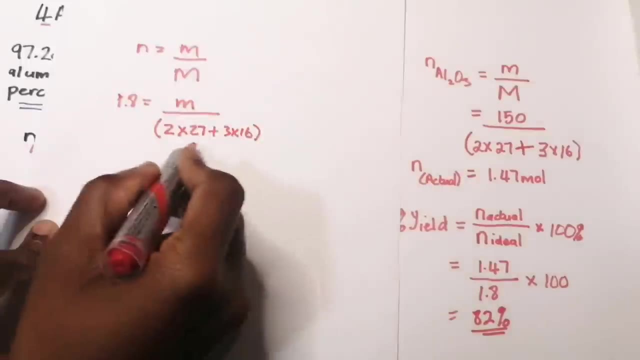 Okay. So in this case, I'm just going to say this is 2 times 27.. Okay, Plus 3 times 16.. Okay, That's our molar mass for aluminum. So what am I trying to do? I'm trying to determine the mass of it. 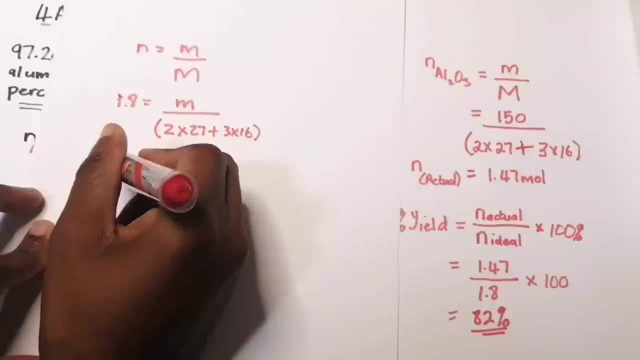 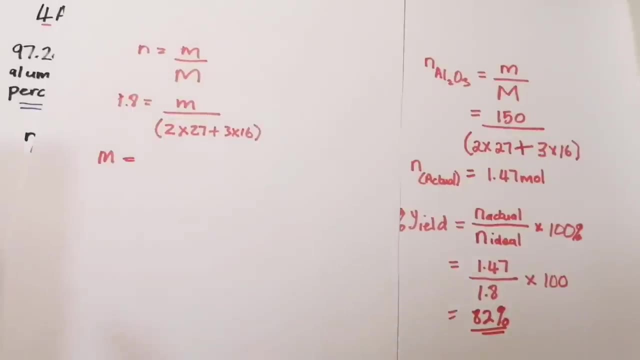 right, So the mass of aluminum we actually produce. Okay, So that would be 1.8.. Okay, So we cross multiply there. Okay, Obviously that's over 1.. So we cross multiply, So our mass is going to be 1.8. 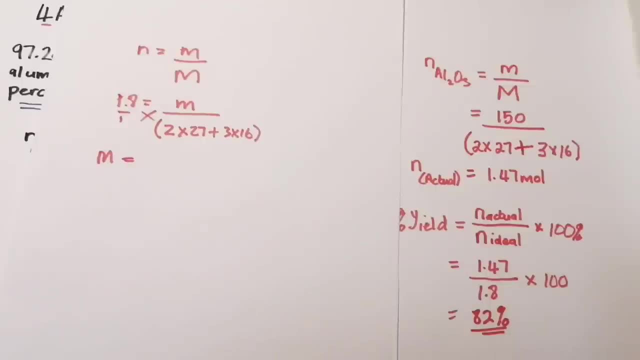 multiplied by so that's 2 times 27 plus 3 times 16.. Okay, All right, I happen to get a. oh no, there's something that I did wrong there. So that's 1.8.. Okay, And so that gives me 183.6.. Okay, So, all right, So I get 183.6.. Okay, So I get 183.6.. 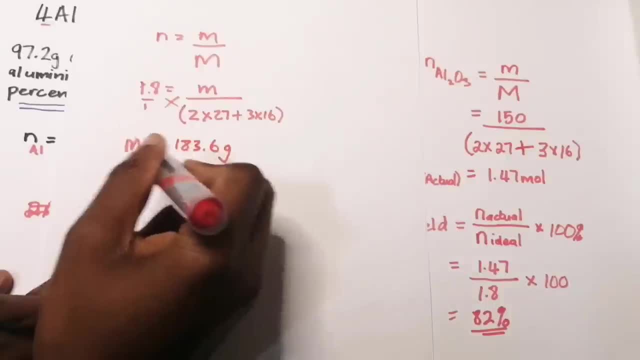 0.6.. 0.6 grams. Now note what are these. These are the ideal. oh, this is the ideal mass. Okay, This is the ideal mass of aluminum oxide that I would have produced. But remember, what do I want? I want to calculate. 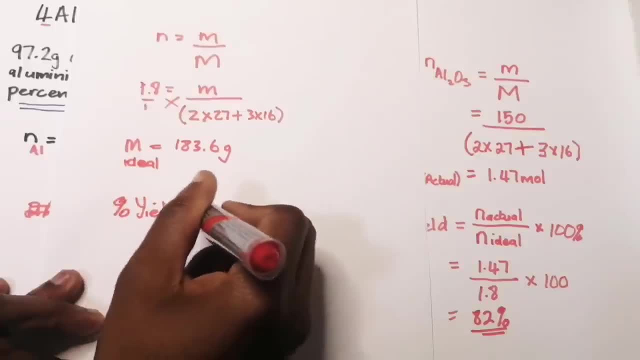 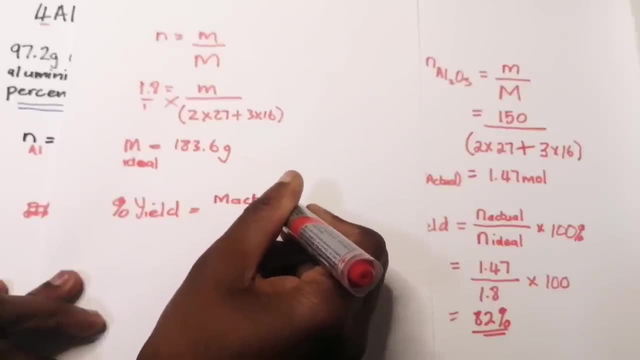 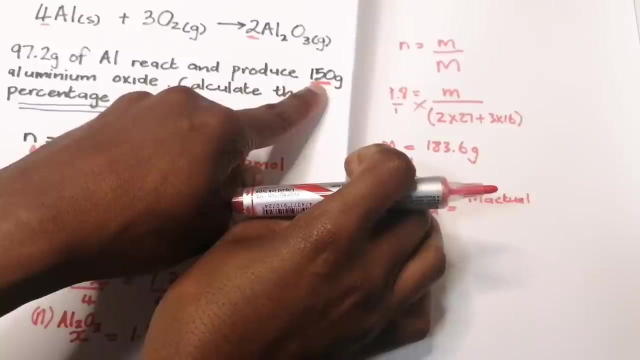 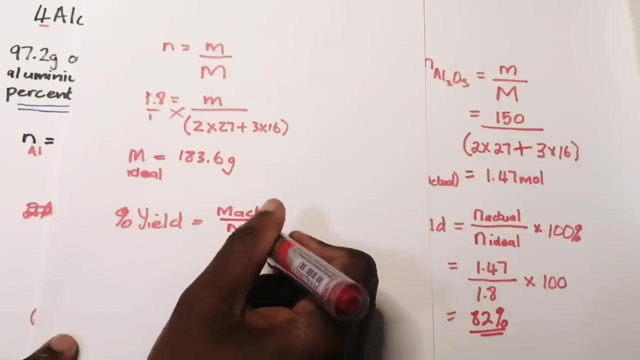 the percentage yield, right, The percentage yield. So, just like we did there, it's going to be Mass, Actual, Right Now. Now, So remember, where do we get the actual mass? It's the one that they gave to us. They told us that we produced 150 grams, right? So it's going to be my actual mass divided by the mass that I would have produced ideally, right. 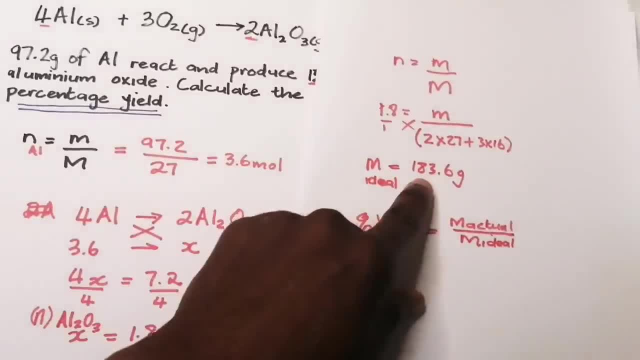 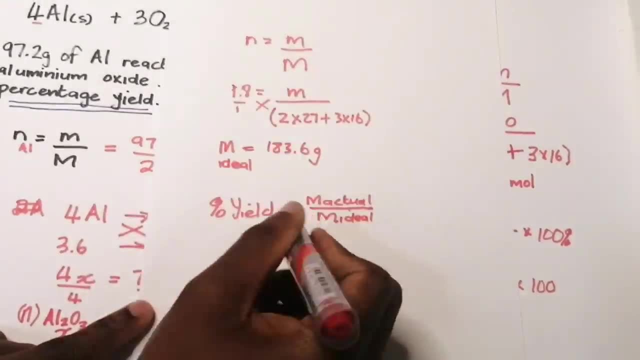 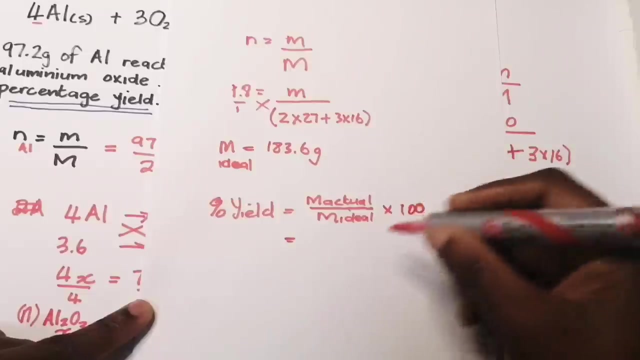 So which one is the ideal mass? It's the one that we just calculated there. Okay, So all I just simply do is multiply it by 100. Please remember that. So that's multiplied by 100. So all we simply do is to say 150 divided by 183.6, multiplied by 100. And I'm quite confident. 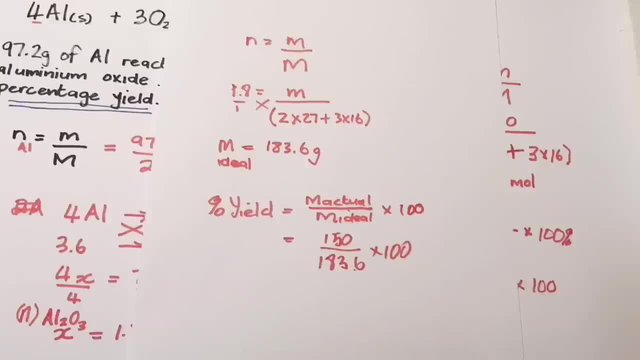 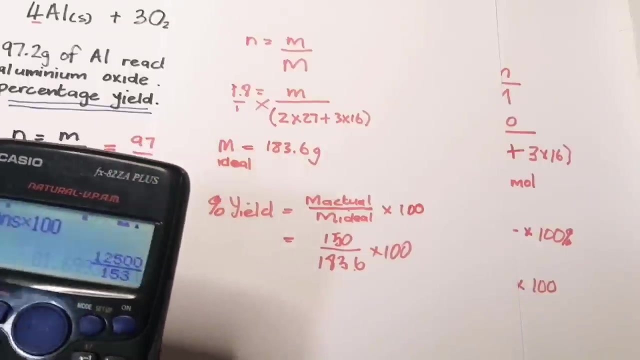 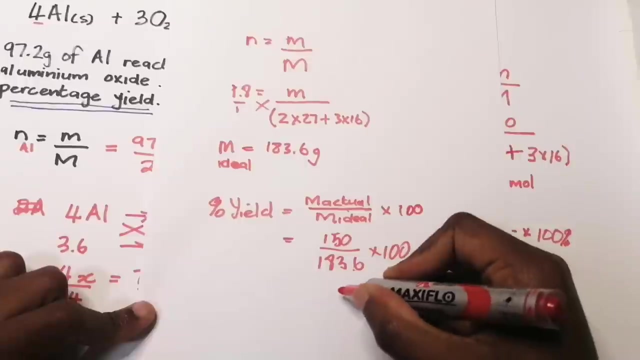 I think we should be able to get the same answer. So that's 150 divided by 183.6.. Okay, I get a sort of similar answer. Multiply that by 100.. Okay, And remember we rounded that off to 82%. So it means that your percentage there should be 82% of the actual yield.